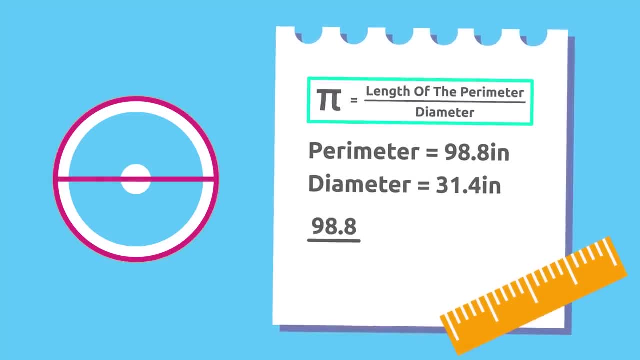 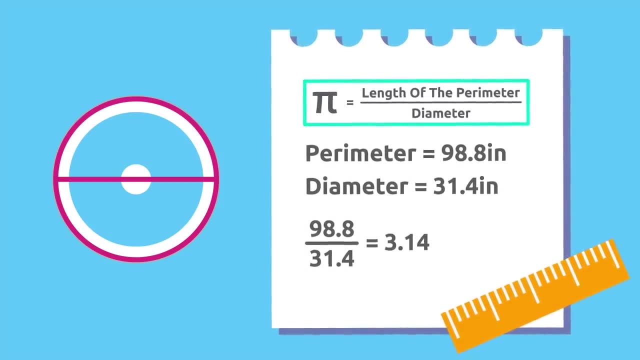 If we divide 98.8 by 31.4,, we'll get 3.14.. Now measure the perimeter of this swimming pool, Or let's say, wave pool. We'll make sure to practice this module for 10 minutes. then take a picture with your takeout boy in the spring and bring it home overnight. Divide the length of the perimeter by its diameter and the result you'll get will be 3.14.. Let's see: The perimeter of this wheel is 98.8 inches and its diameter is 31.4 inches. 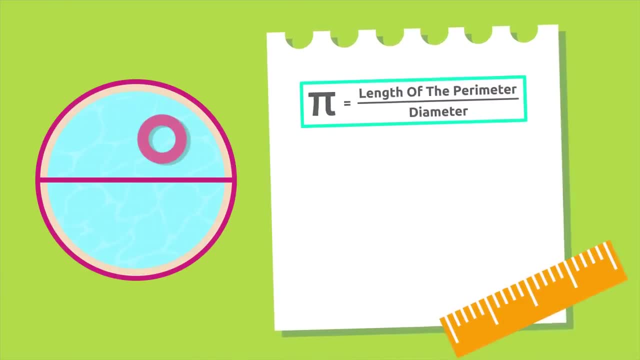 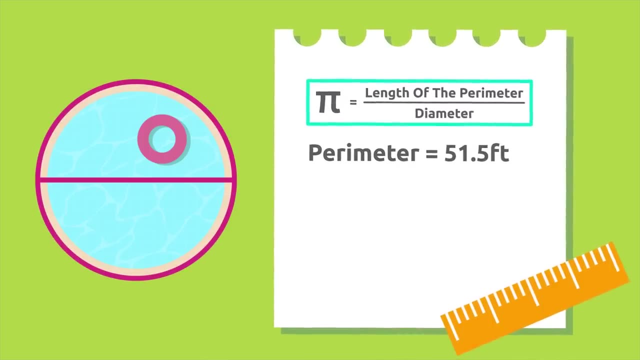 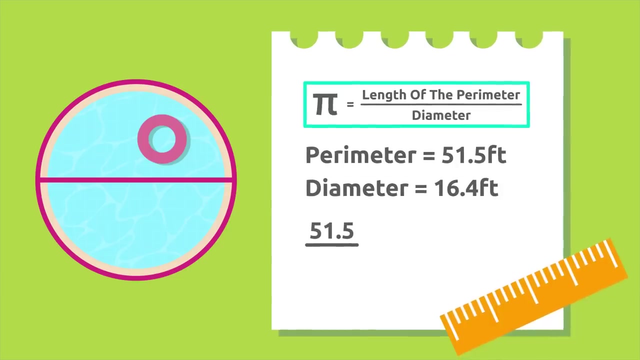 Divide the length by its diameter and you'll also get 3.14.. Let's see: The perimeter of this circular swimming pool is 51.5 feet and its diameter is 16.4 feet. If we divide 51.5 by 16.4, we'll get 3.14.. 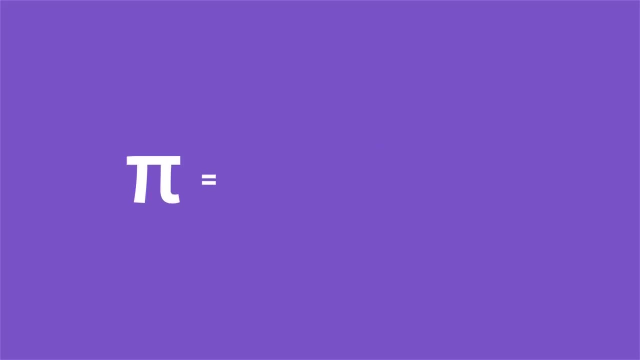 It's like magic, isn't it? The result we get every time we divide the perimeter by the diameter of any circle in the world will always be 3.14.. This happens because pi is a mathematical constant. In other words, it's always the same number, regardless of what the circles or circumferences. 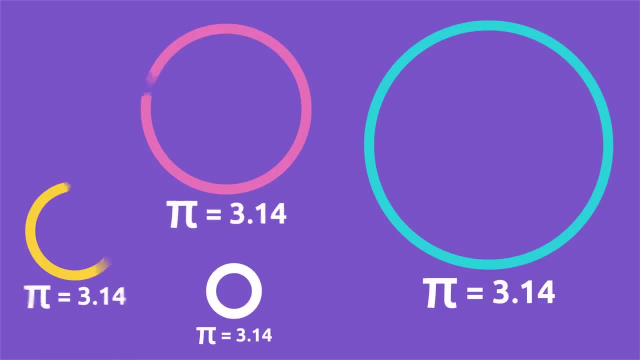 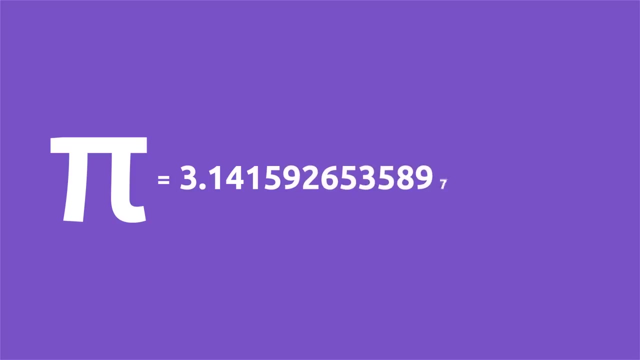 may measure. There's a very interesting fact we haven't told you about yet: Pi is represented by this Greek letter and it's an infinite number: 3.14.. 1, 4, 1, 5,, 9,, 2, 6, 5,, 3, 5,, 8,, 9,, 7, 9,, 3, 2, 3,, 8,, 4,, and the digits go on forever. 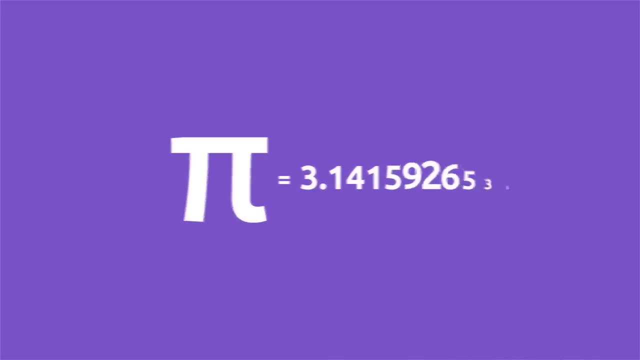 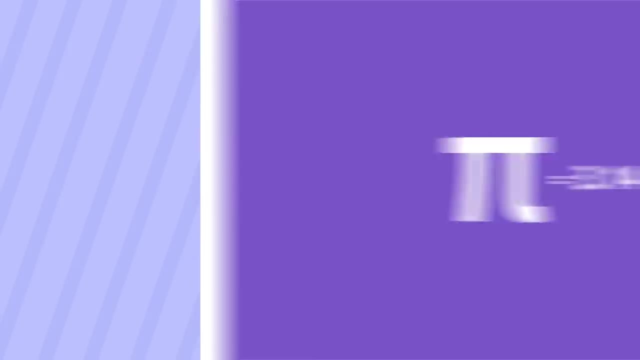 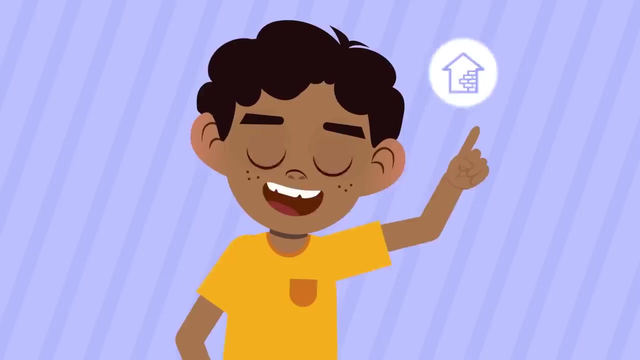 and ever. In everyday life, this number is shortened to 3.14 to be expressed in a simple way and make calculations easier. Today we learned that number pi is one of the most important mathematical constants. Any architecture, mechanics or engineering projects wouldn't be possible without the. 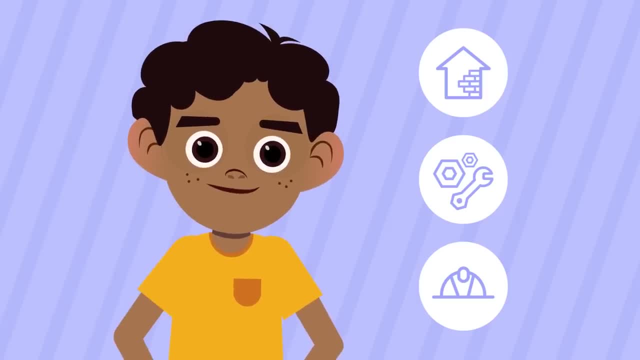 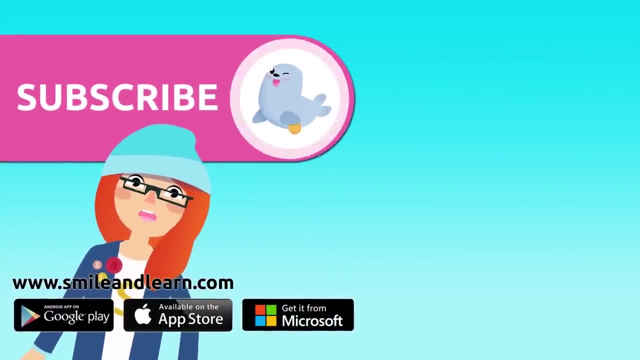 number pi. Did you like the video? We have so many more. Subscribe by clicking on the seal Ah, and if you want to keep watching more videos, click on the boxes.